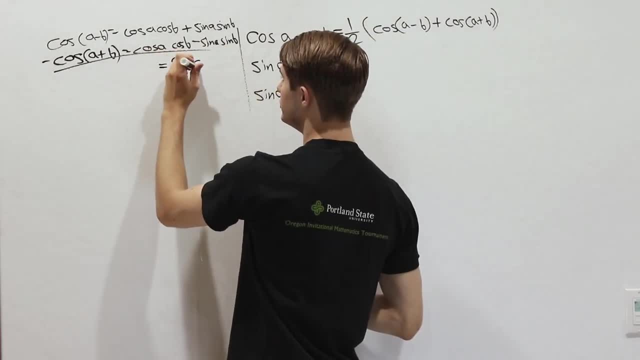 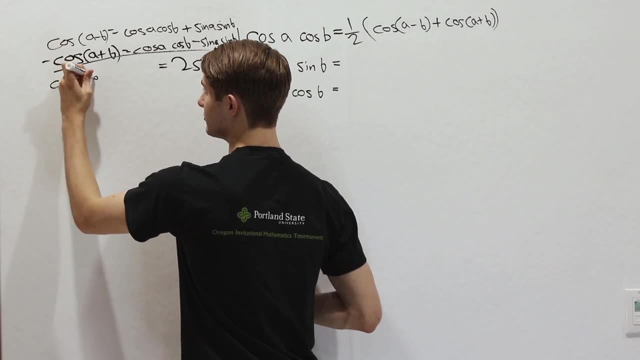 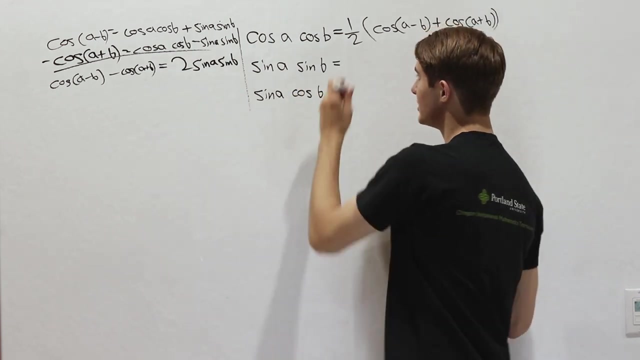 and we're going to end up with on this side of the equation: 2: sine a sine b. Okay, Then on the left side we get cosine a minus b, like before, and then minus cosine a plus b. So we go over here. if we want to take sine a sine b by itself, we get 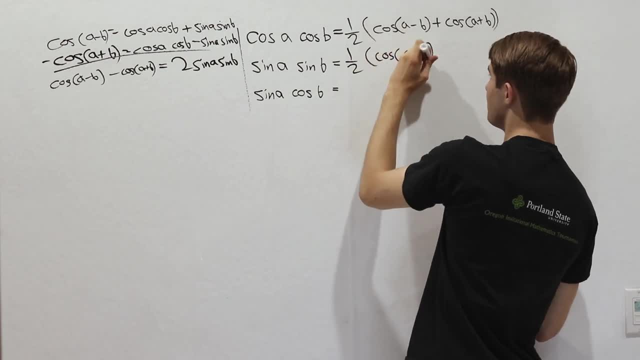 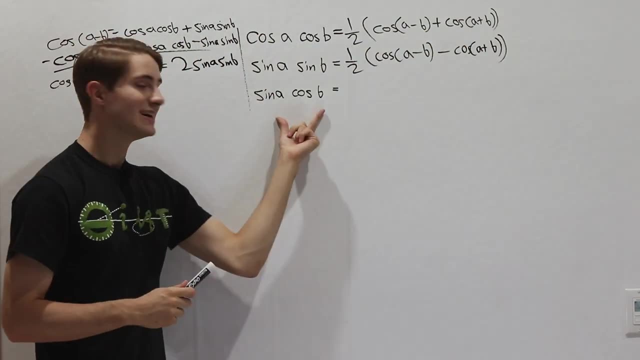 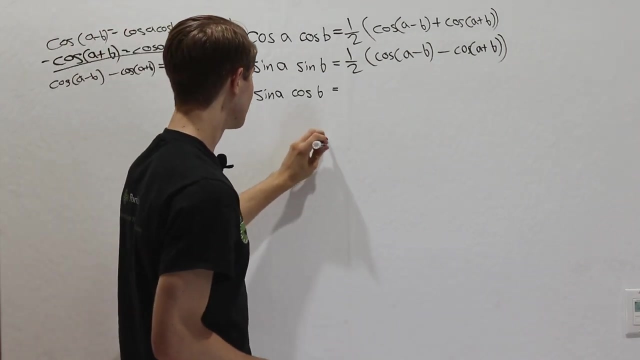 one half cosine a minus b minus cosine a plus b. So the last one we want to do right here is sine a cosine b, And in order to do that we'll need the angle sum formula for sine. So if we take a look at this sine, 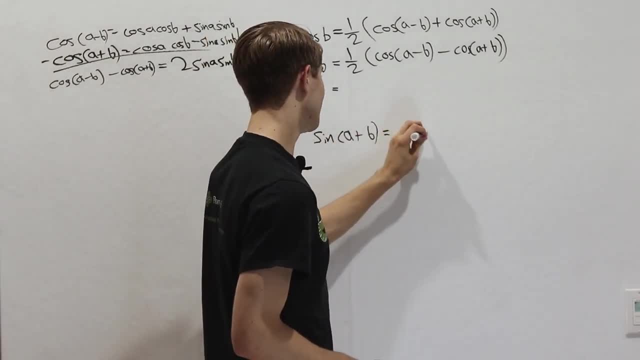 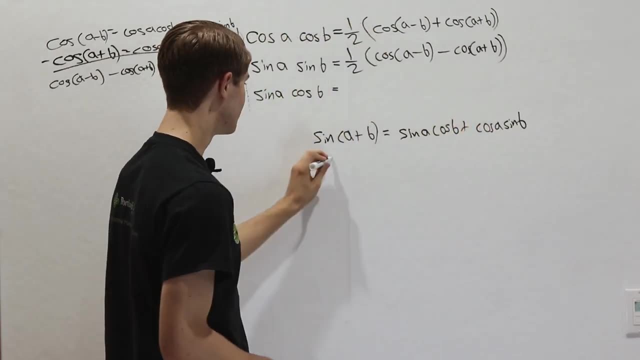 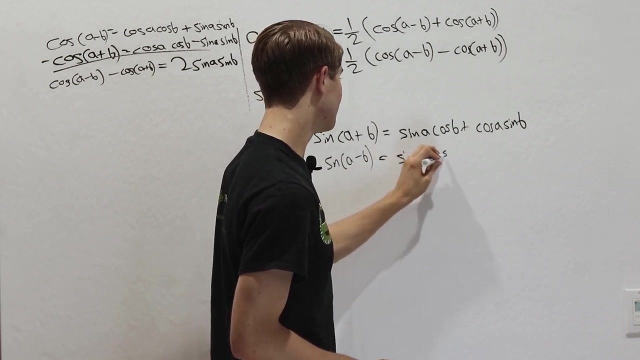 llega to sine a sine a plus b. Well, that's going to be sine a cosine b plus cosine a sine a plusb. Then if we do sine of a minus b, just like we did with the cosine, we'll get sine a cosine b, like before, and then minus cosine a. 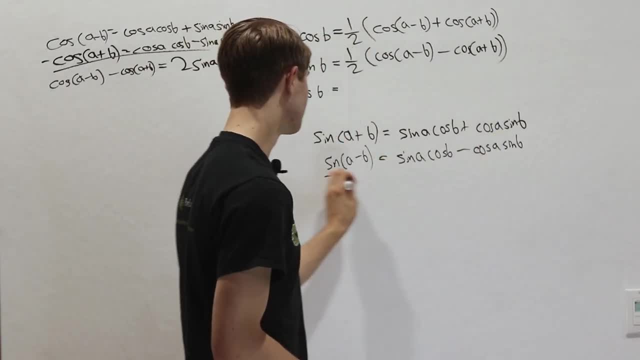 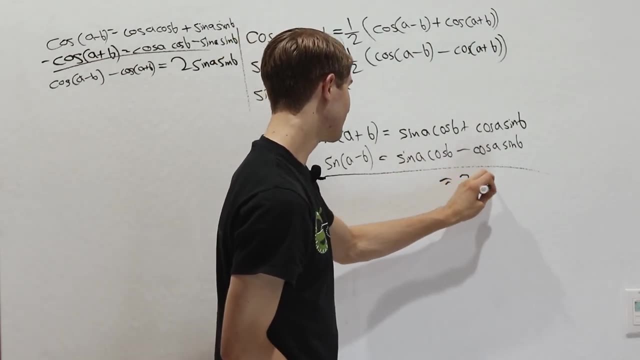 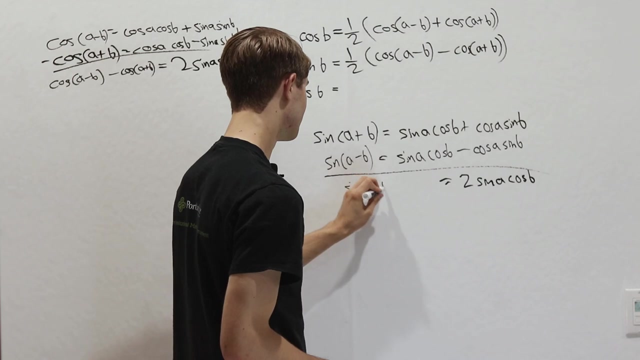 sine b. So again we add these two equations up. these cosines a sine b terms are going to cancel out, and over here we're going to get two – sine A cosine B. On the other side we'll get sine A plus B, plus sine A minus B, just like that. 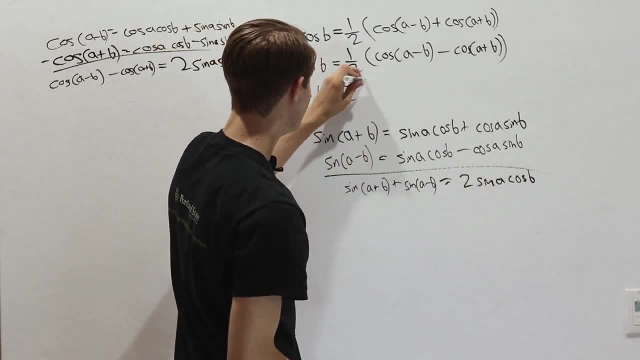 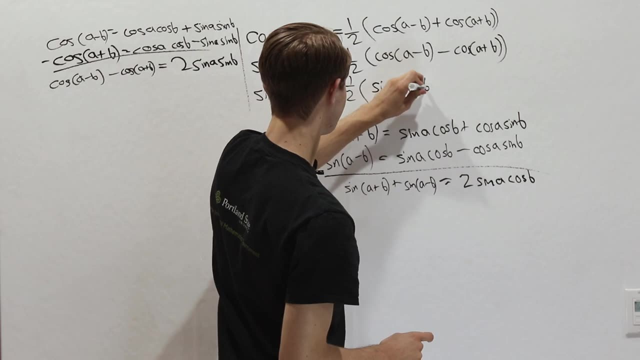 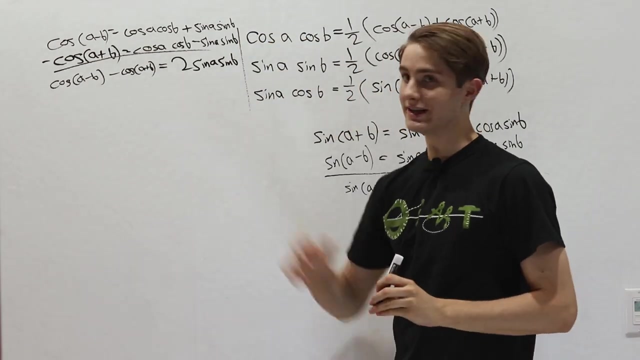 Now, if we want to isolate sine A cosine B, we'll again take a half And for the sake of making all these equations look the same, I'll write sine A minus B first and then plus sine A plus B, So using the angle sum identities, just like this, and adding the A plus B and A minus B versions. so 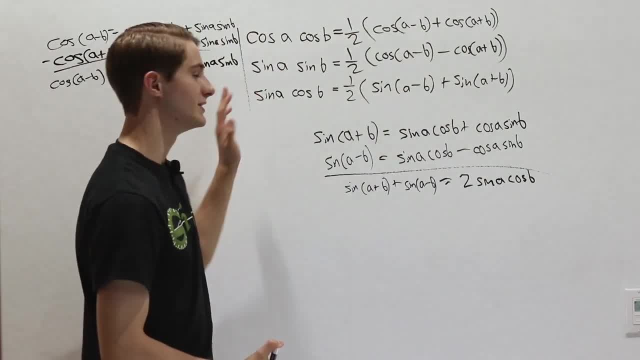 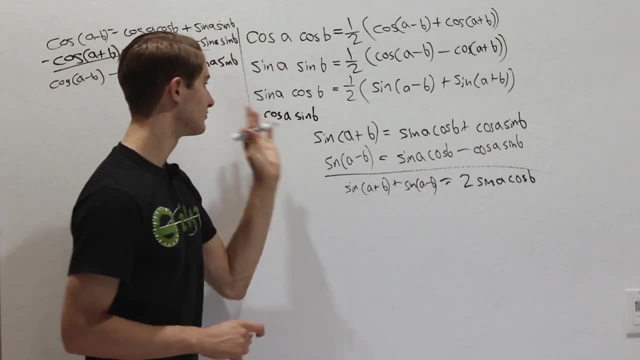 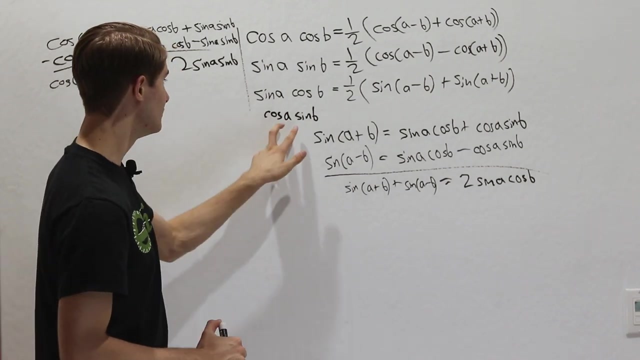 that each part of the equation cancels out. we can get these three identities. Now some people might be asking: what happened to cosine A sine B? Isn't that the fourth thing that we should have on our list right here? And the answer is: if you find an expression in this form, all you have to. 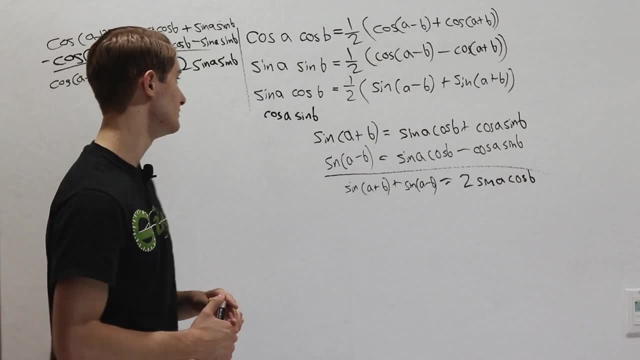 do is flip these two terms around, because multiplication is commutative, and then you can just apply this same identity right here. There's no reason to add in a new identity if we already have the information we need right here. So these are the product-to-sum formulas for sine. and cosine.